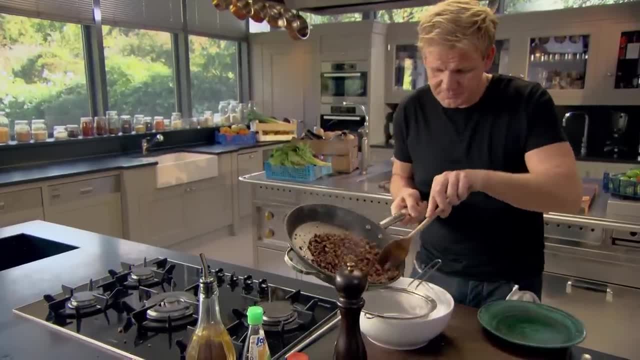 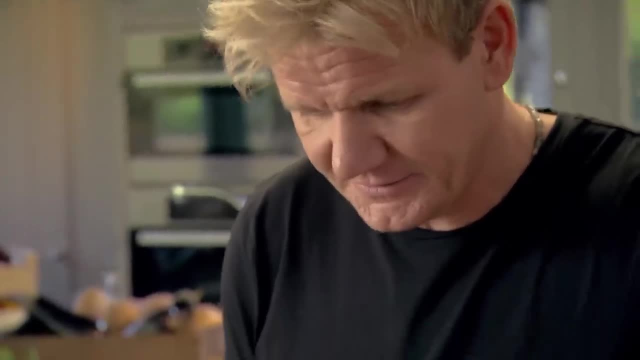 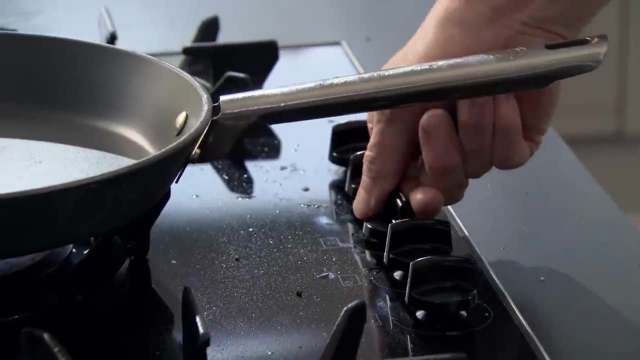 crispy Smells incredible And draining. it is crucial. It keeps the mince nice and crispy and you get rid of that excess fat. That's lovely. Now just wipe out the pan and wash it Low gas. Now we're gonna add texture to the. 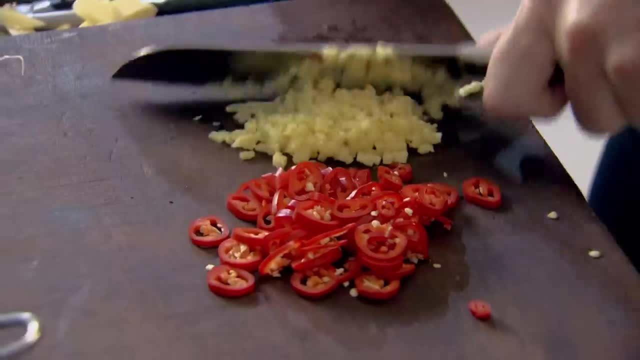 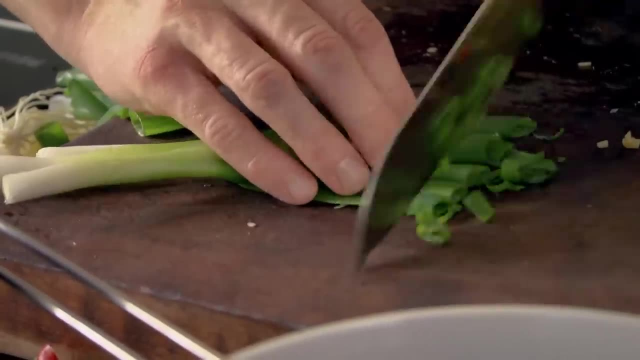 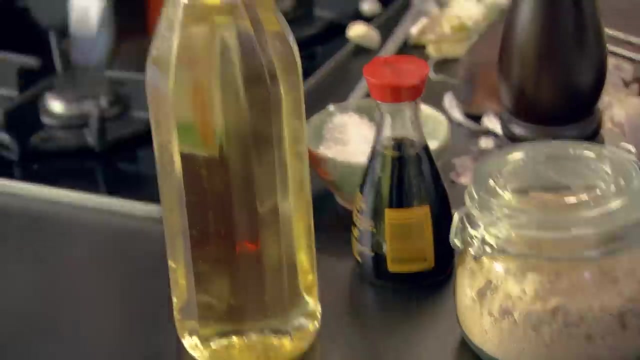 mince Finely chopped chilli, ginger, garlic and spring onions. Spring onions give the sort of mince a really nice freshness because it just gives that crunch Nice and thinly. Now we'll fry off the chillies, the ginger, the garlic first. 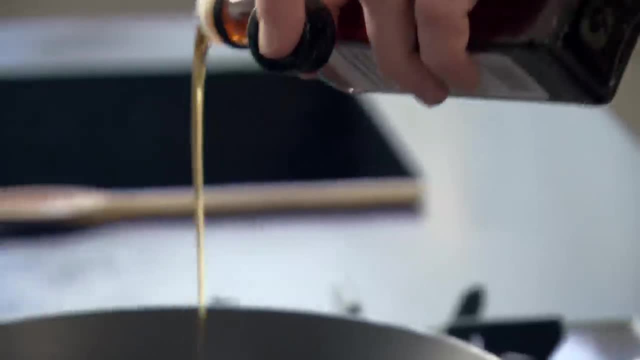 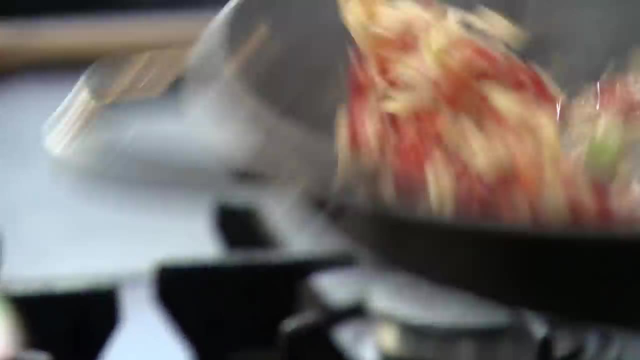 Sesame seed oil Teaspoon. only in Garlic, chilli, ginger in. Fry that off nicely. The sesame seed oil just lifts up the whole flavour Touch of brown sugar That starts to really caramelise the chilli, the garlic and the. 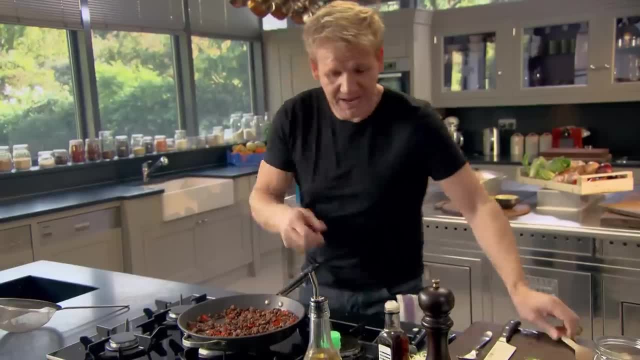 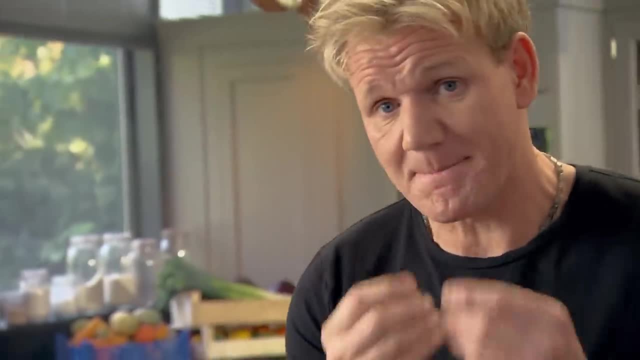 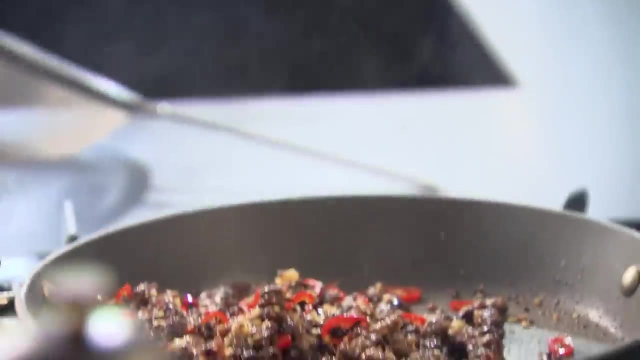 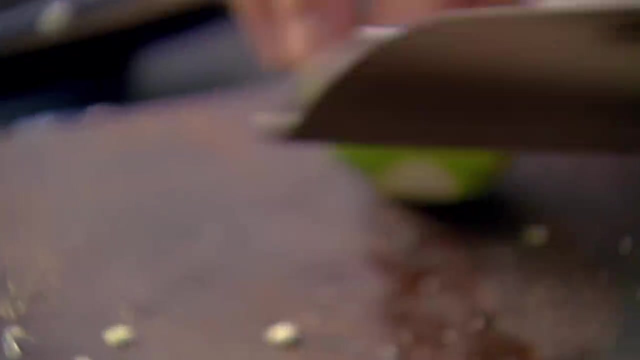 ginger Mince in, Now my fish sauce. That gives it the saltiness. You can see now why it was so important to get that mince really crispy, because nothing's going soggy, It's staying really crispy. Fresh lime, That makes the mince fragrant, And then lime juice Roll. 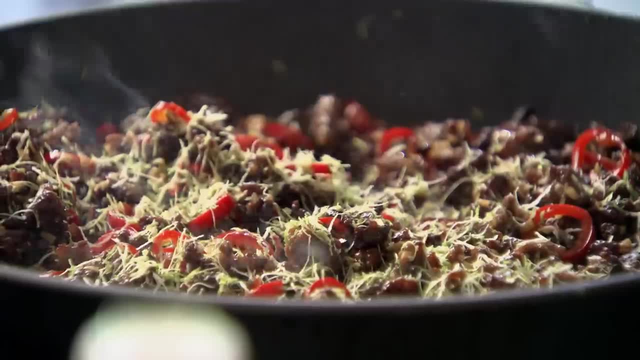 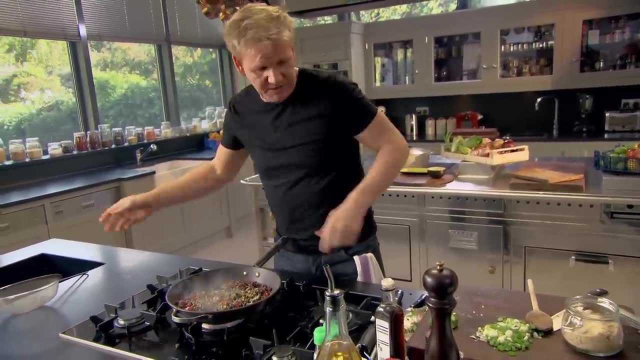 it And squeeze that in there. Incredible. I've got a salty, I've got the heat, I've got the sweetness, and now I've got the acidicness as well, and then, finally, my spring onions in. Let it marinate Right at the last minute. 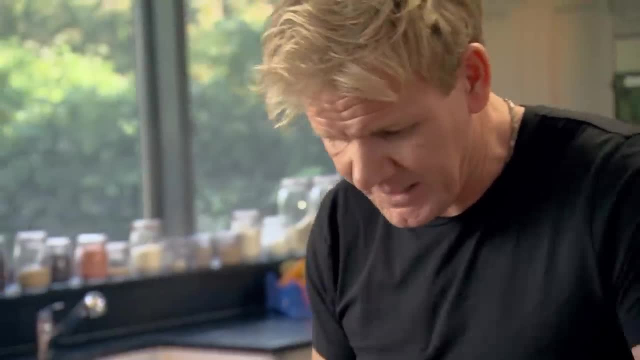 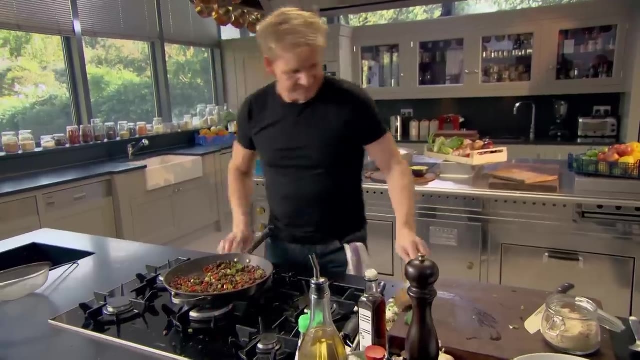 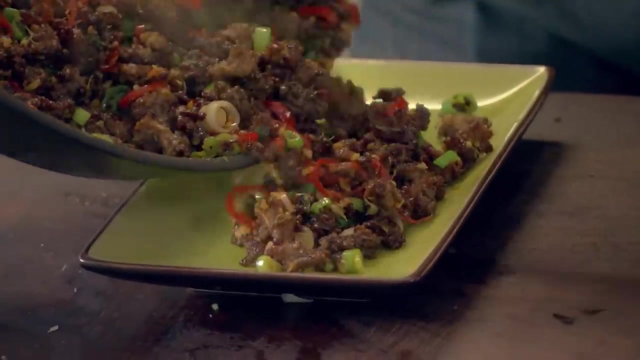 so I've got crunch in there as well. Smellsamazing, Literally cooked the mince now, with sort of thirty seconds to go Gas off, Take it out Lovely, Ta-da, Lovely. Looks incredible, Smells so inviting. 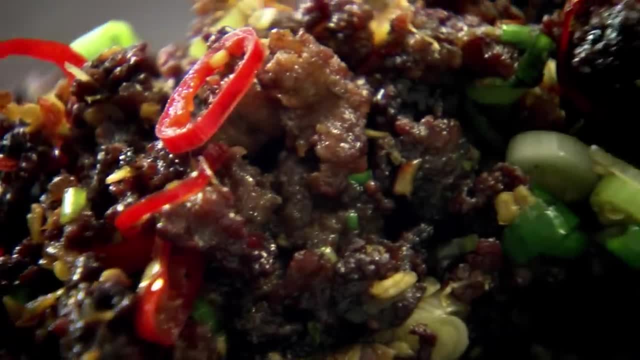 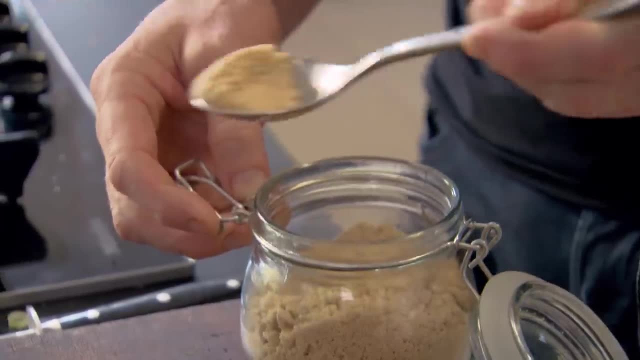 To go with the chili beef. I'm making a simple, sweet and spicy dipping sauce so everyone can dress the crispy mince to their own taste. Dipping sauce: a little teaspoon of the brown sugar, soy sauce gives it a nice sort of dark, rich color. 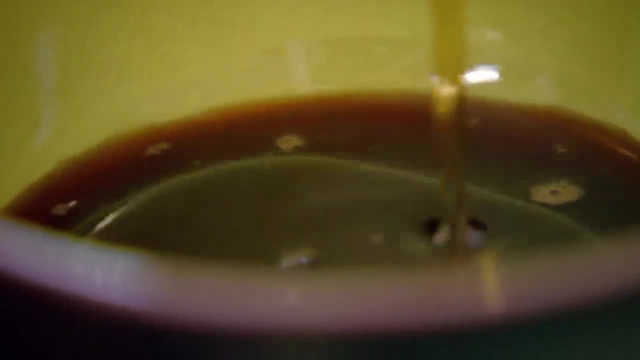 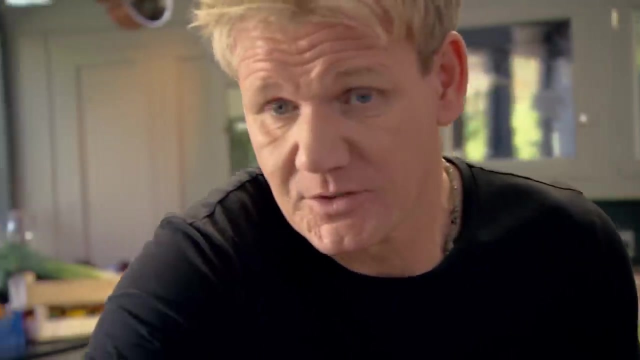 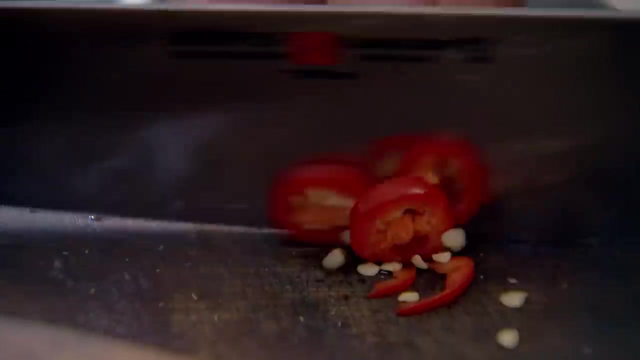 Sesame seed oil a tablespoon, And just top that up with a tablespoon of olive oil. That stops the sesame seed oil becoming too rich. A teaspoon of fish sauce and then a touch of chili. Leave the seeds in again. Want the heat in that sauce? 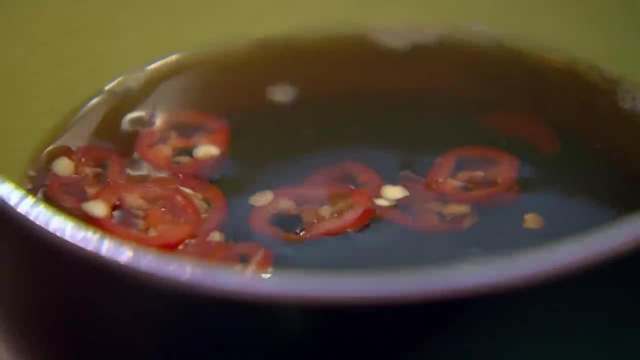 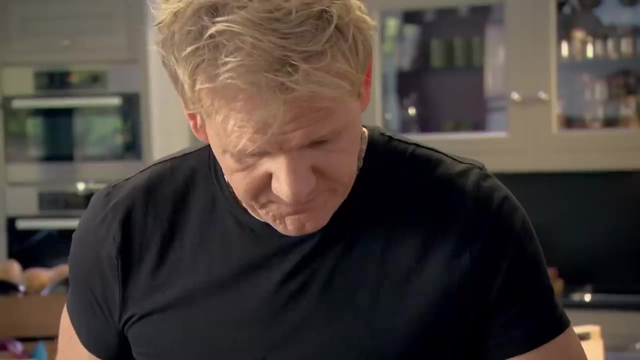 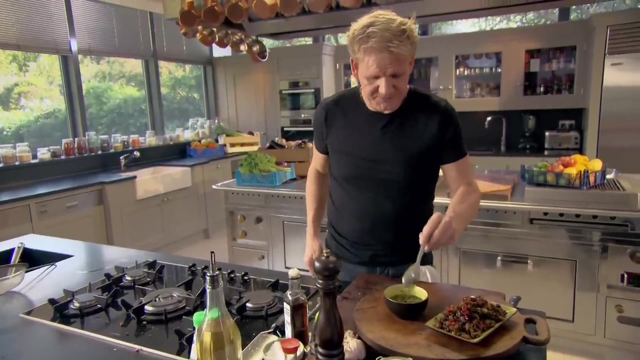 So impressive, an amazing show-off centerpiece. Lime juice in and the coriander Chop it through once. Give that a little mix up. Just check the seasoning. Mm, that's lovely, That's enriched. Now the lettuce. 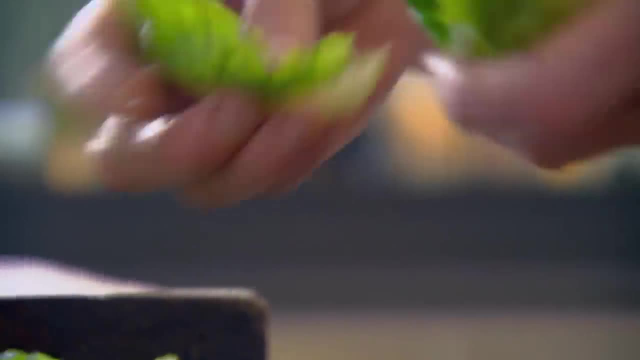 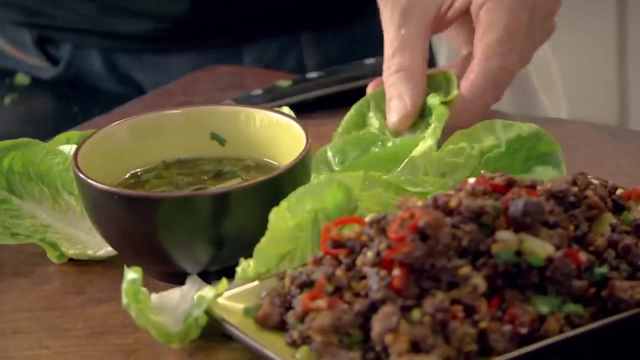 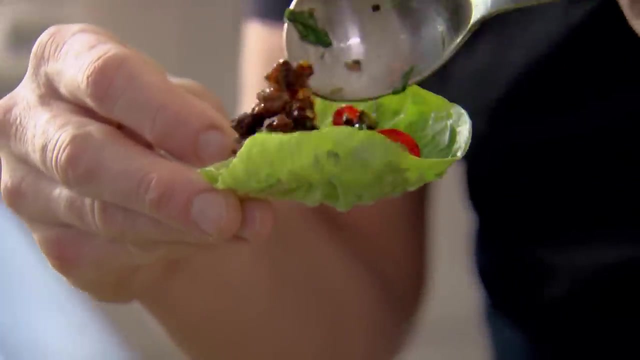 I'm going to use baby gem because it's really nice and durable and sort of quite strong. So you just sort of sit these nice trimmed lettuce leaves around. Now the exciting part serve. Take your lettuce up, spoon in your mince. 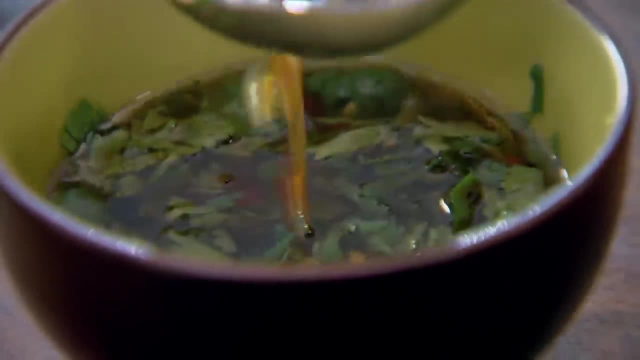 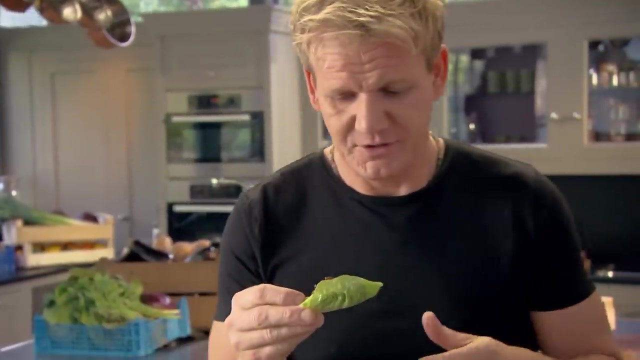 And then a little touch of dressing, Just a little drizzle. Nice, And that's the secret of having good, easy, relaxed food: is that You just help yourself. Food that looks and tastes a million bucks doesn't have to be complex. 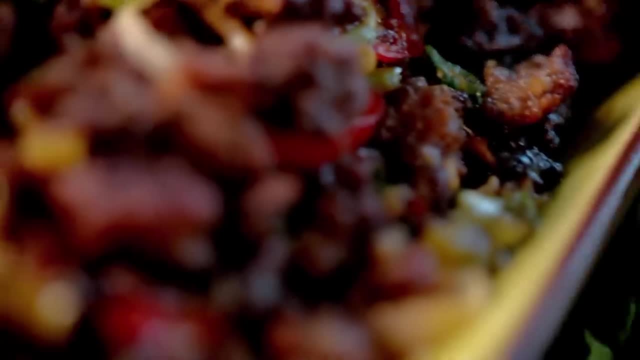 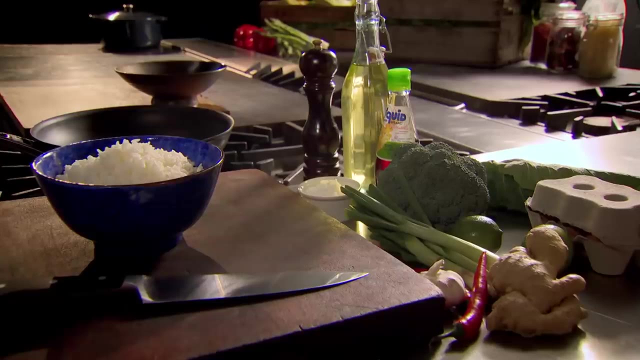 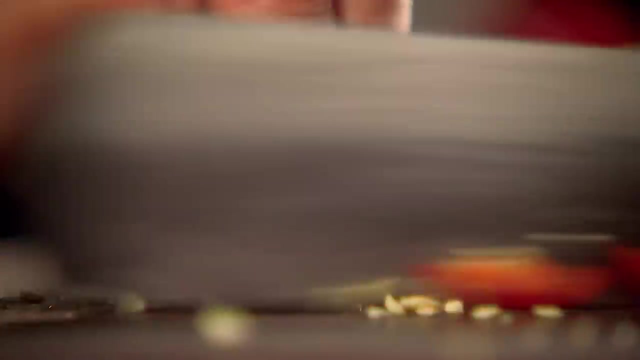 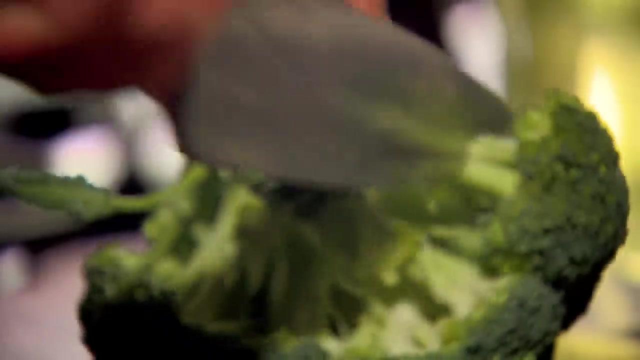 This dish is as fun to cook as it is to eat. First, get prepped: Chop garlic, ginger and chili, keeping the seeds for extra kick. Slice spring onions, Chop spring greens And trim a head of broccoli. Then whisk two eggs. 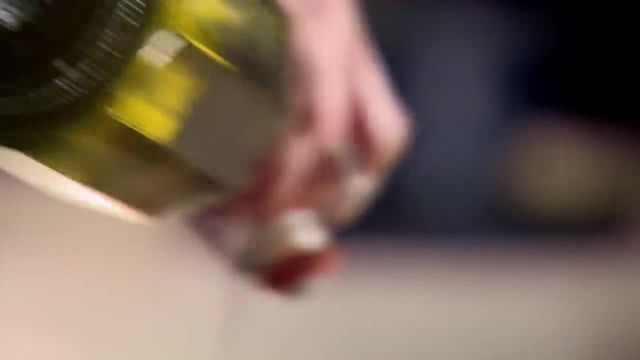 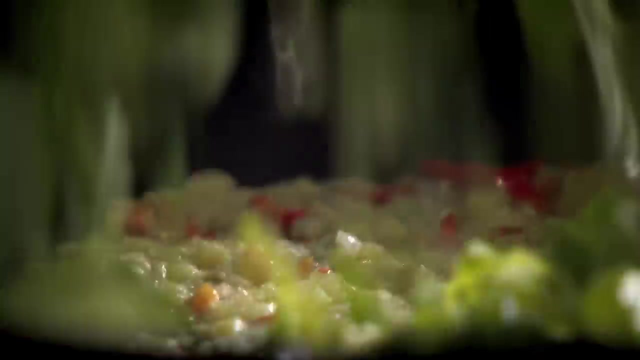 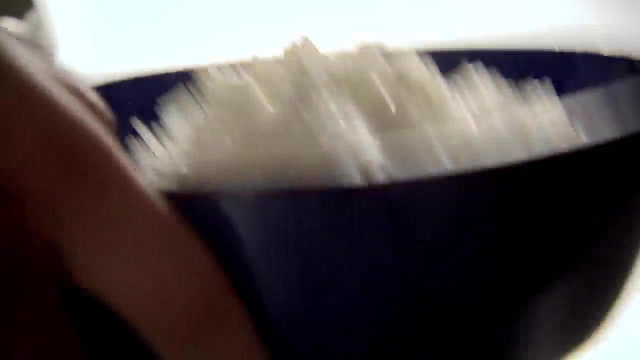 Prep done, Stir fry on. Add a good glug of oil to a hot pan: Garlic, ginger, chili, Next the spring greens and broccoli. Add water to steam, Then cook rice. This dish is perfect for using leftover rice. 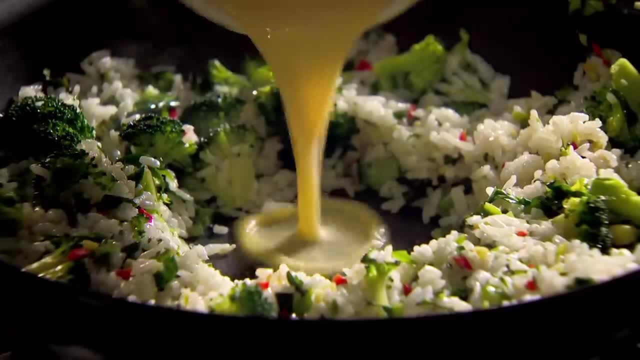 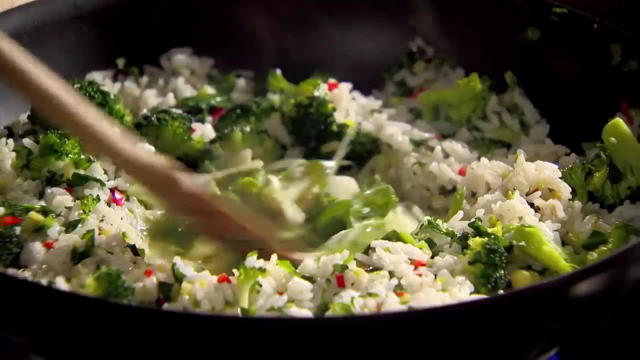 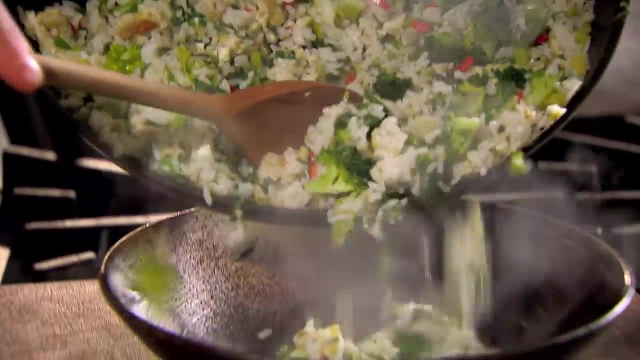 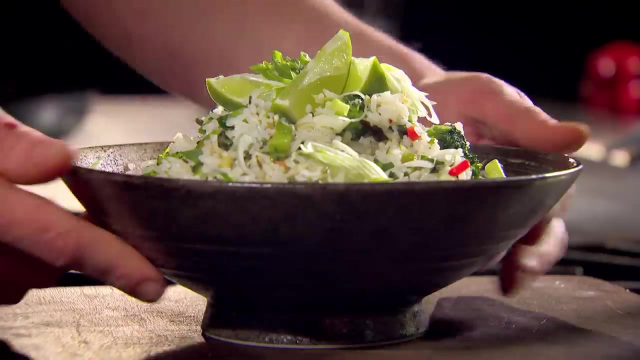 Come on, Make a well. add the eggs, spring onions and a dash of fish sauce. Scramble, then mix, Season, Top with lime and spring onions. My fragrant fried rice, made simple with advanced prep and ready in five minutes. 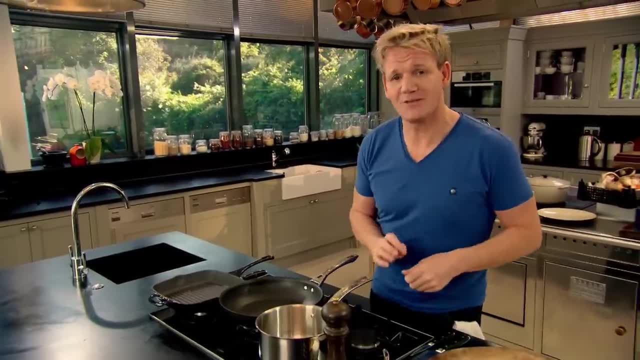 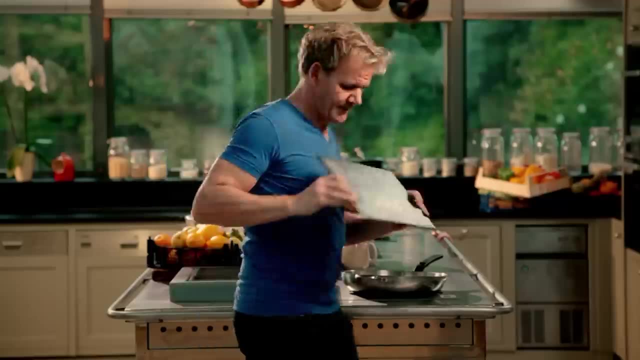 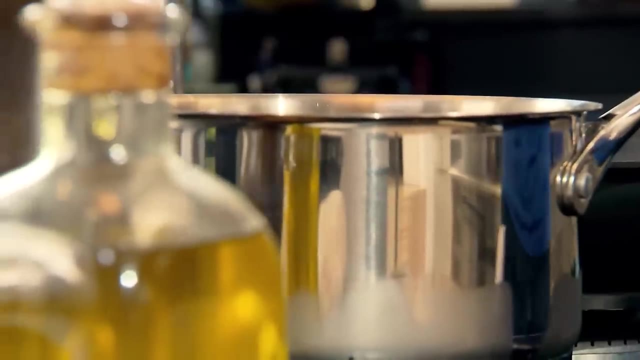 This fantastic, fast and simple pasta dish, made with everyday ingredients, just goes to prove you can eat good food whenever you want. Really important to put the water on first so you can just have it gently simmering away, ready for the pasta. 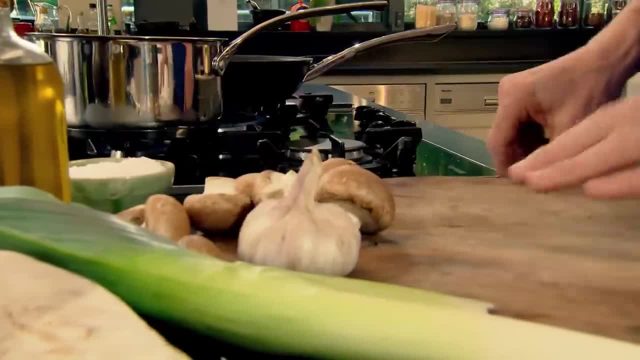 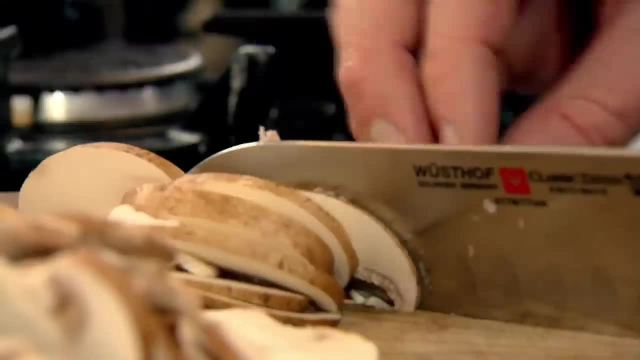 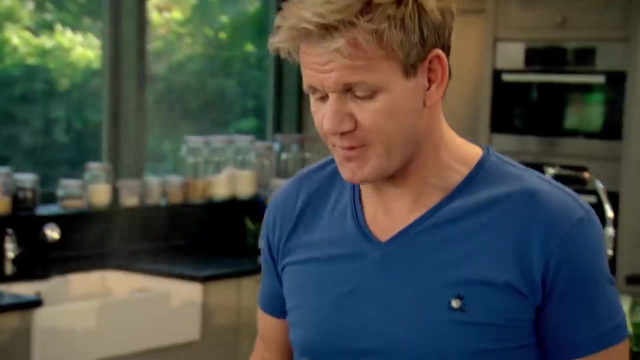 While the water comes to the boil, start the sauce by slicing mushrooms, First off fingers, One in front, two behind, Up and down. Then add olive oil to a hot frying pan. I want that nice colour on the mushrooms. Off the heat literally ten seconds. 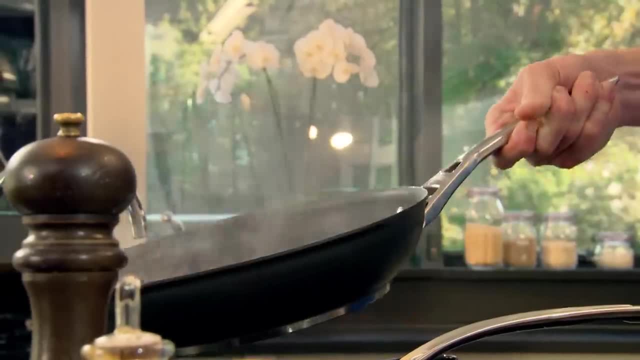 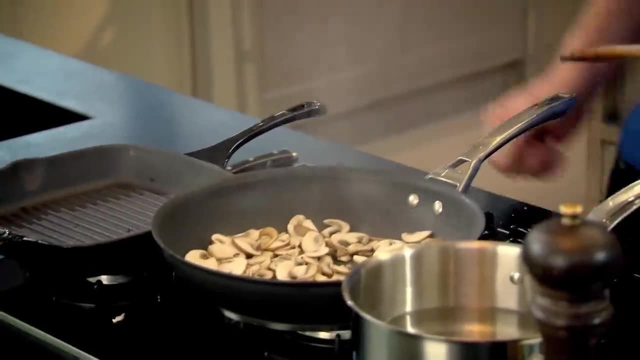 And when you toss something really important to get all the ingredients at the end of the pan, Push down and pull back. That noise that ssssss. that's all the water coming out of the mushrooms. Next, finely chop a fat clove of garlic. 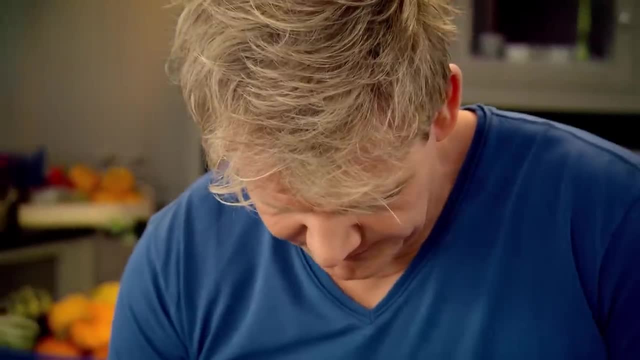 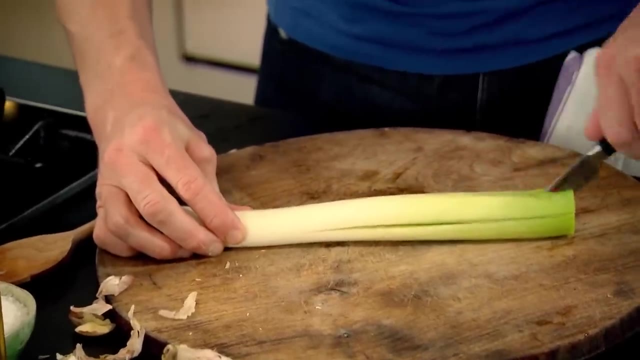 Then prepare your leeks. Just take your knife and go down through the centre, turn it over and again into quarters, So you've got all that opening up, And then just rinse the top of that to get rid of any potential dirt or sand. 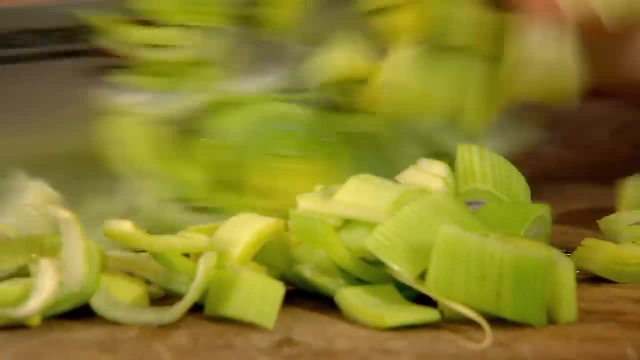 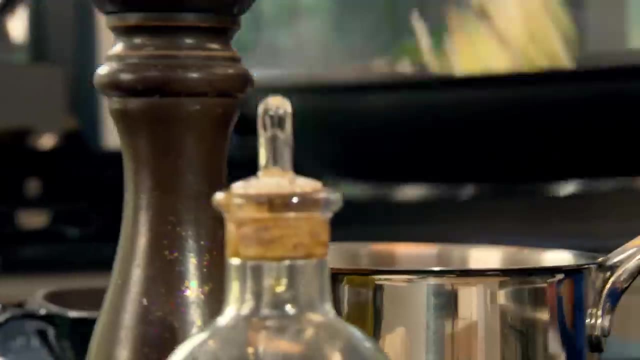 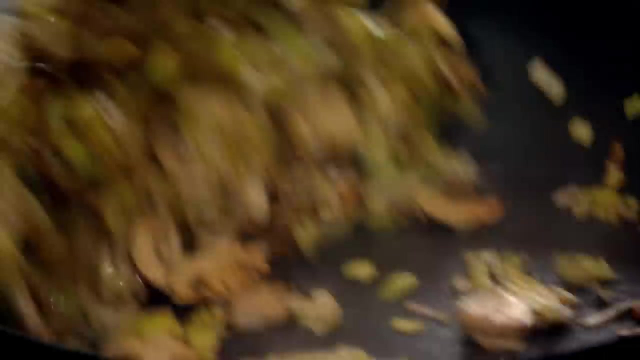 It just breaks up into nice little quarters, Add all that leek into those mushrooms- Beautiful. And now the secret is to get rid of that water inside the leek As it cooks down. all the water's gone and you've just left that really nice, intense flavour. 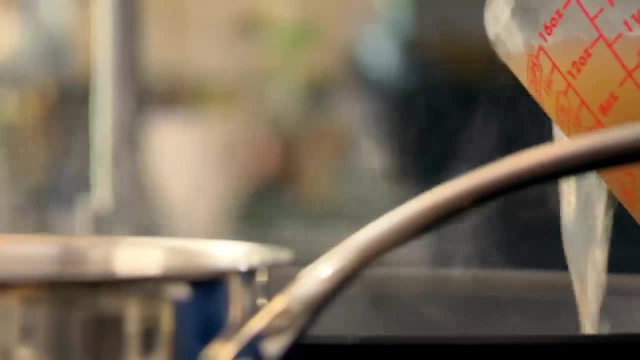 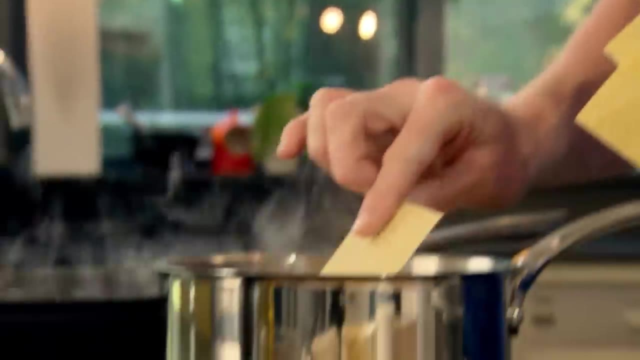 Garlic's gone, nice and crispy. Now we're going to add a touch of chicken stock in there. Mmm, beautiful Lasagne sheets. Just going to drop the sheets in to the water. Lasagne sheets are an unusual choice for a dish like this, but they work brilliantly. 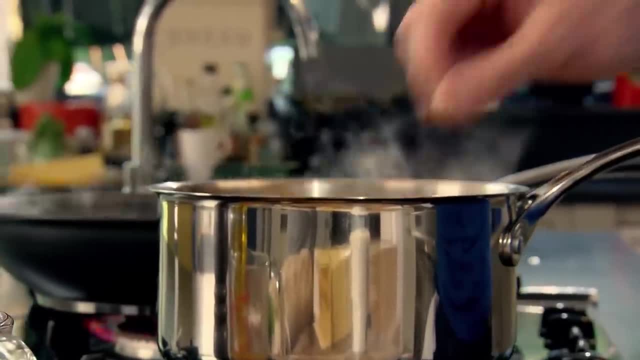 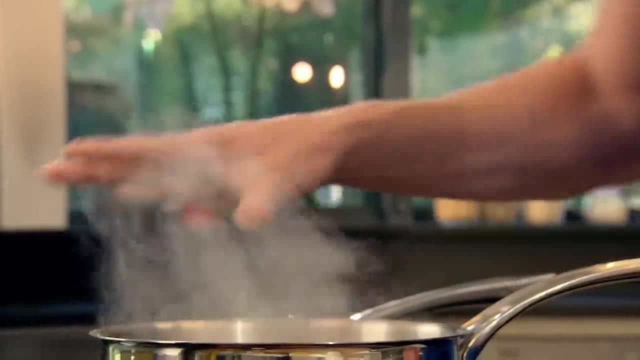 Although any type of pasta you've got in the cupboard will do, And just twist that pan. That stops any pasta actually sticking to the bottom of the pan. That stops any pasta actually sticking to the bottom of the pan. Chicken stock will reduce down by half. 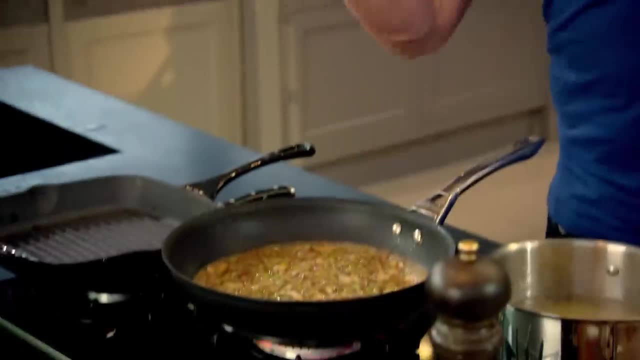 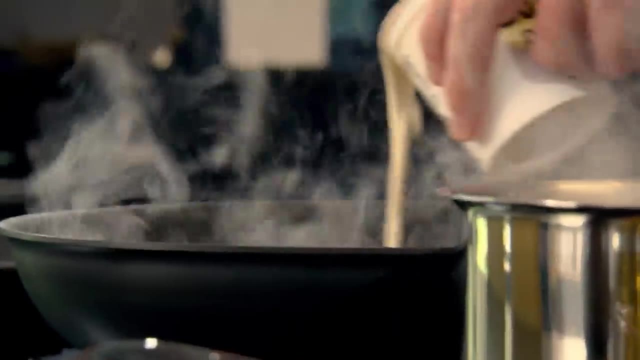 And it's almost glazed. the bottom of the pan Basically washed all that wonderful flavour off. Turn the gas down And add a couple of tablespoons of cream. And add a couple of tablespoons of cream. This just enriches the dish. Bring it back up to the board and let it simmer for three to four minutes. 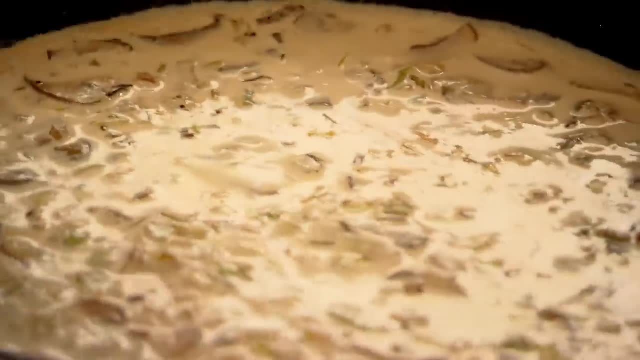 Bring it back up to the board and let it simmer for three to four minutes. Now, the secret of the pasta is just taking it out a little early. Now, the secret of the pasta is just taking it out a little early, So you've got that nice texture. 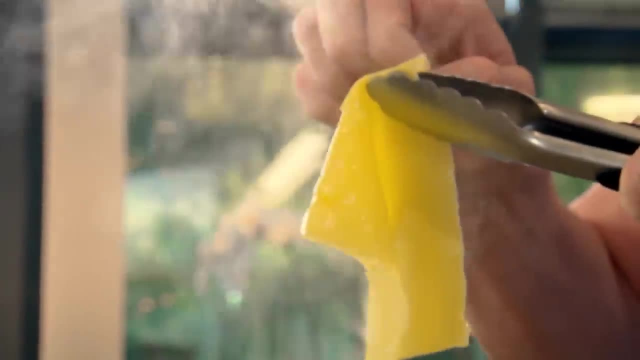 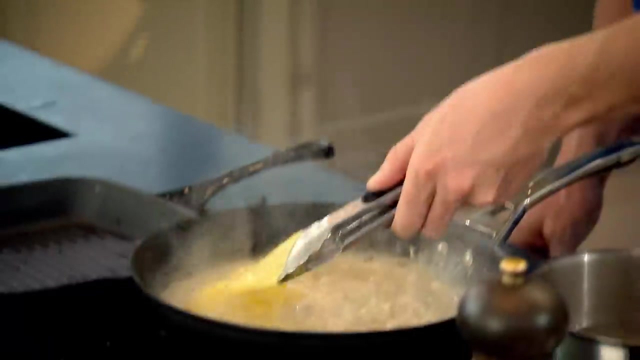 Hold up the sheet and just nip it And you can feel your fingers in the centre. And you can feel your fingers in the centre. It's ready. Turn the sauce down and lay these beautiful sheets and lay these beautiful sheets. 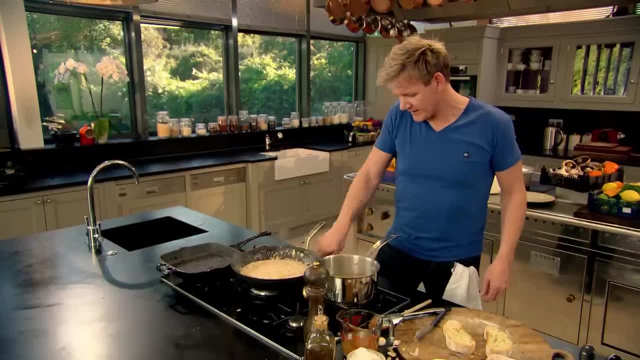 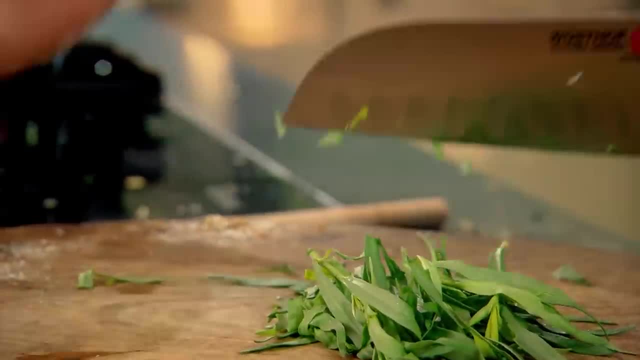 of lasagne into that sauce. I'm just going to turn the gas off now And let the pasta sit in there and absorb that amazing sauce. Finish with chopped fresh tarragon. Finish with chopped fresh tarragon. It's a delicious herb. it goes brilliantly well with mushrooms and leeks. 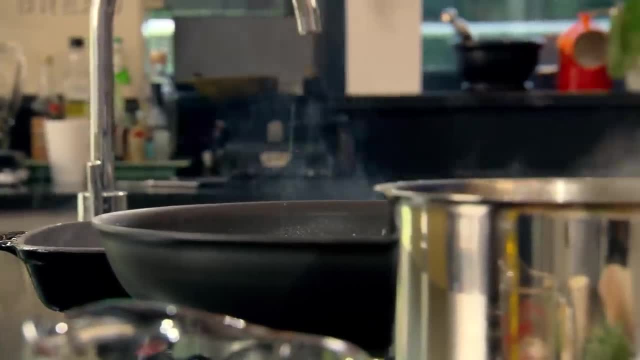 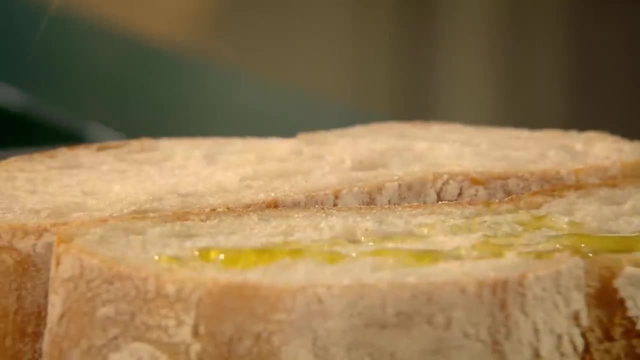 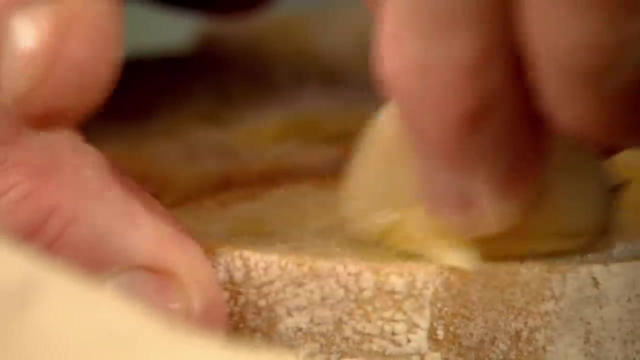 Just let that sit Almost. sort of infuse To serve. I'm making a quick bruschetta To serve. I'm making a quick bruschetta, Two nice slices. drizzle that in olive oil, A little bit of garlic, Just rub the bread. 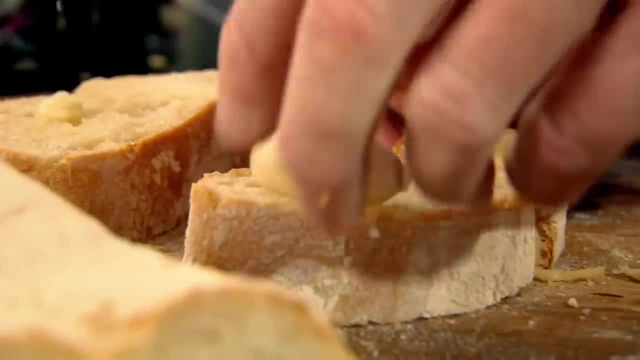 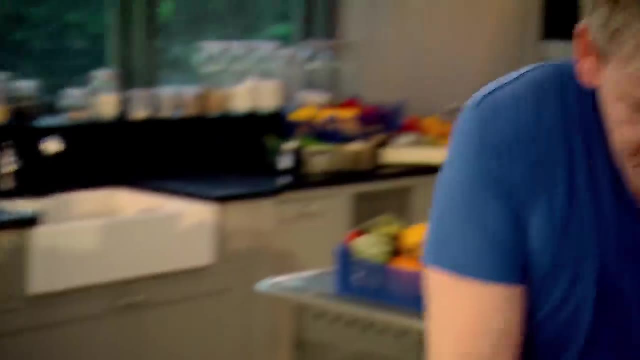 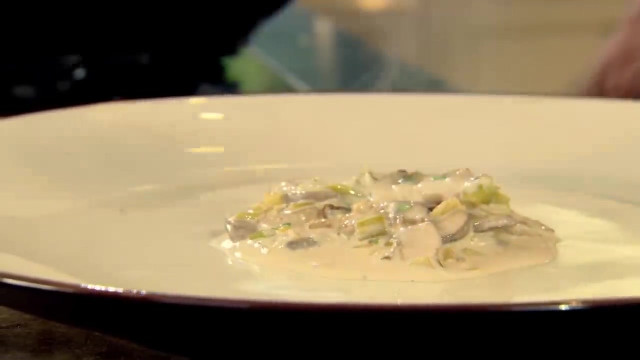 The crust as well. the crust is what really takes that garlic. Now pan for the bread a little touch of olive oil As it starts to smoke bread in. But look at the pasta now it's been stained by that amazing sauce. 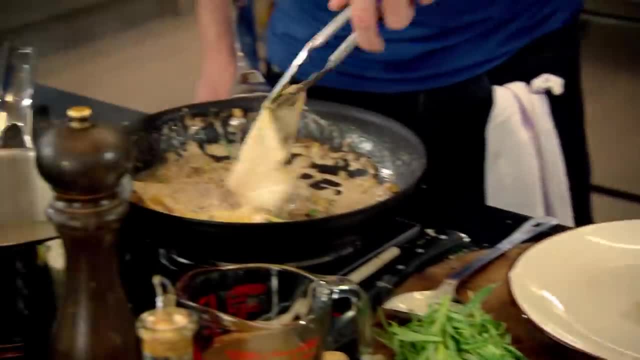 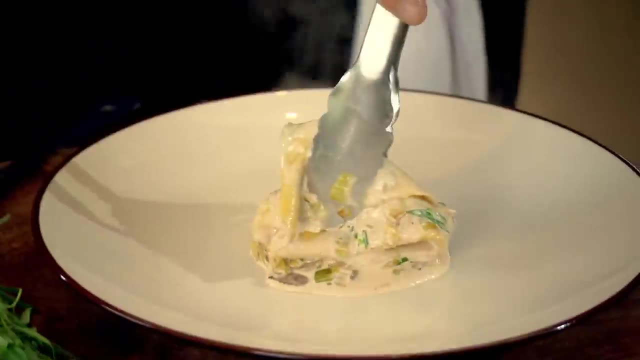 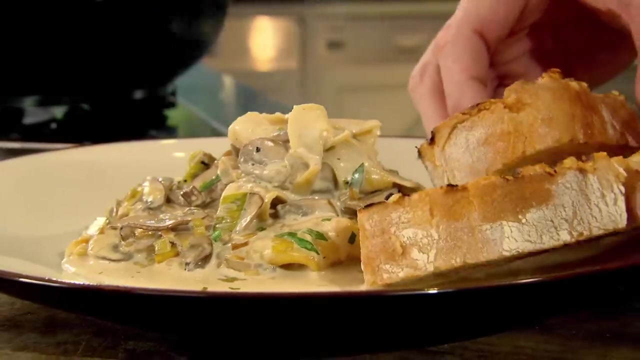 To serve. I want a nice spoon of my mushrooms, leeks and cream. then I'll take my pasta, just twist it and let it sit on top. That tarragon has just lifted everything Bread on, And that's the beauty about something so simple. 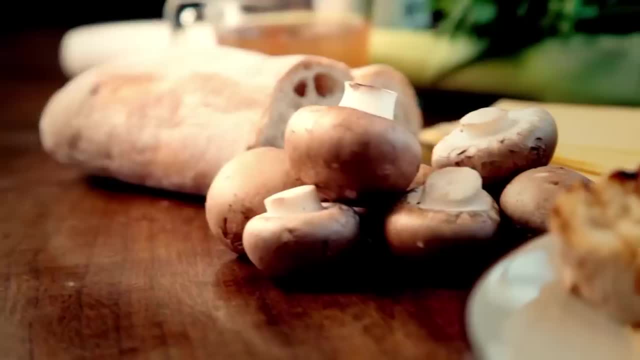 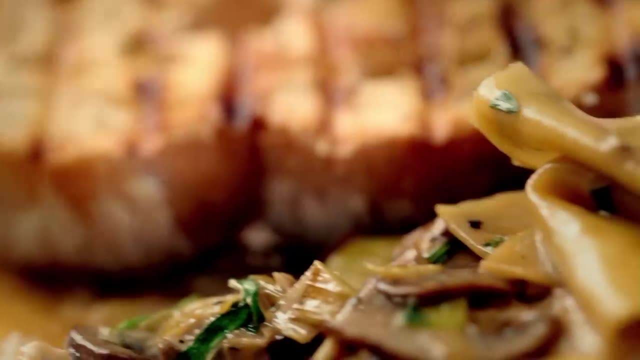 they can be done in 20 minutes with everyday ingredients. A stunning pasta dish. Adding easy and versatile dishes like this to your repertoire is what cooking at home is all about, So you can always make great tasting food at the drop of a hat. 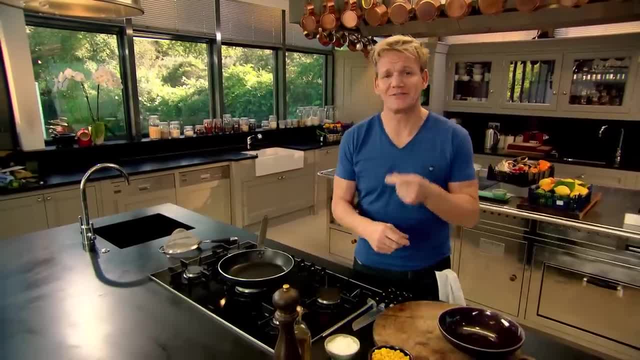 It's brilliant to have a number of great recipes up your sleeve to rely on and, let's be honest, we've all got a tin of sweet corn somewhere, so I'm going to show you how to make the most amazing fritter. 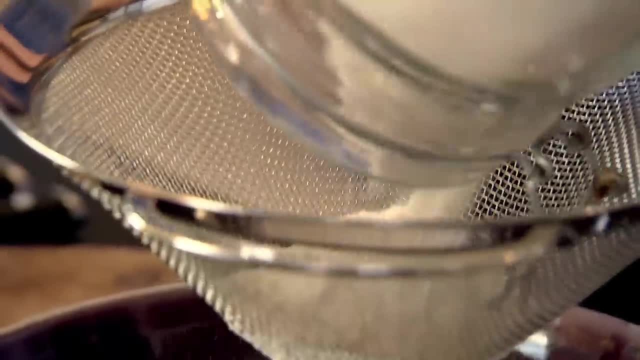 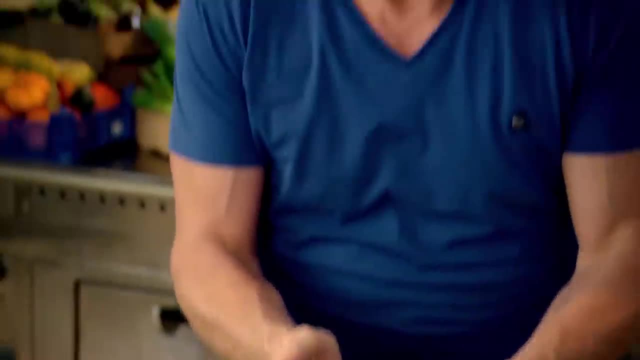 First off the mixture. Take your flour sieve. Really important to sieve the flour. That stops the mixture from having any lumps in there Just like that. Just before you get to the end, I want to put half a teaspoon of baking powder. 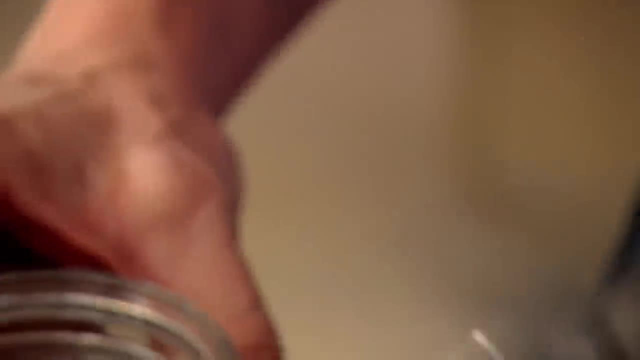 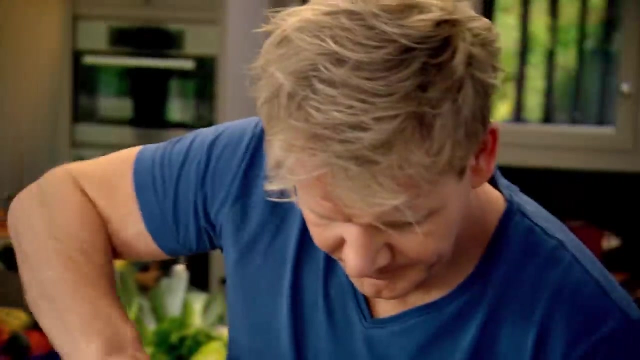 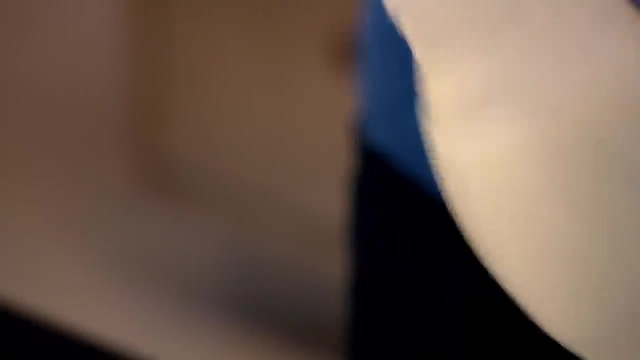 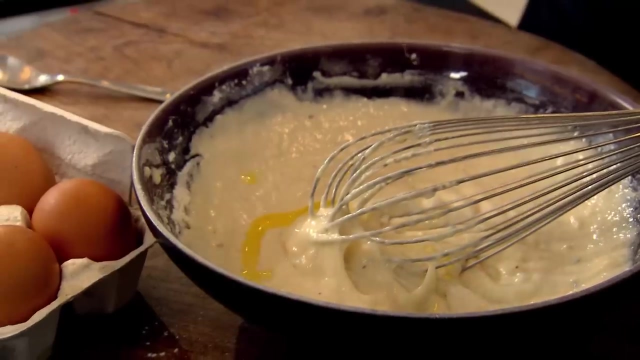 The baking powder gives the mixture some lift In and just sieve that through A touch of salt and pepper. Next an egg And about four tablespoons of milk And give that a little whisk. Now just put a little drizzle of olive oil in there. 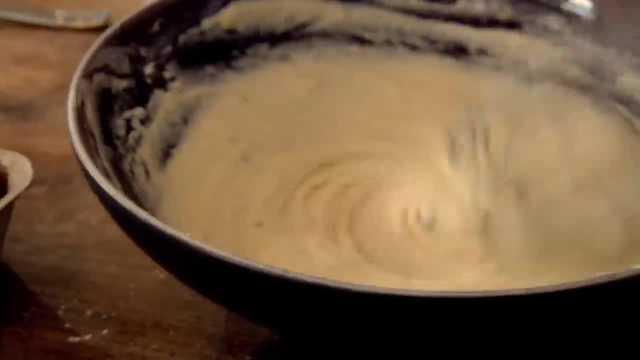 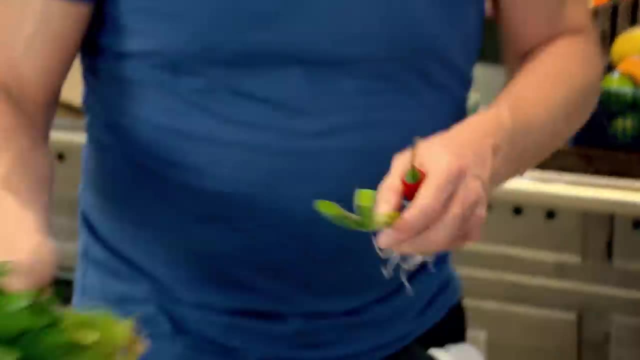 Helps to relax the mixture. Whisk that in. Make sure you've got rid of all those lumps. So look, I want a nice, smooth, almost like a cake mixture. Okay, Next, take the seeds out of a chili to lower the heat. 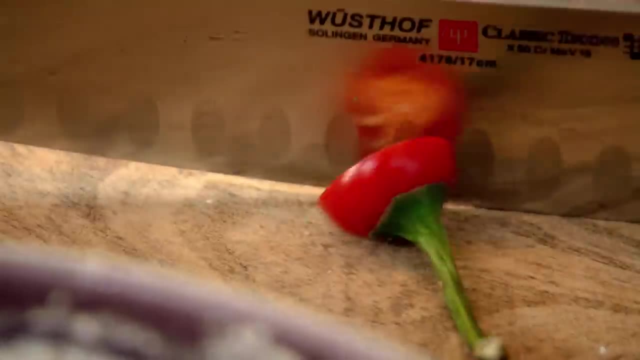 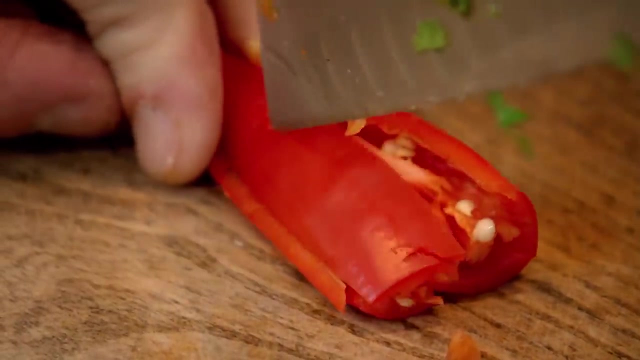 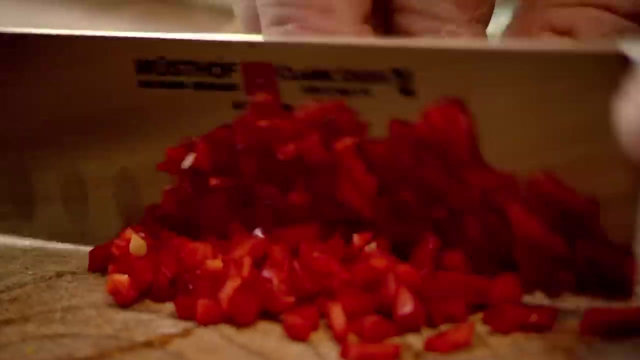 Roll the chili, so give it a really good shake. Tap them out, Slice in half into quarter, And each quarter in half, And chop through. It's a really nice, quick way of slicing a chili Into the mixture Spring onion. 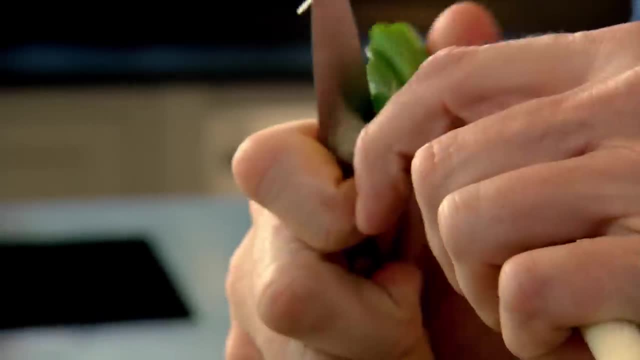 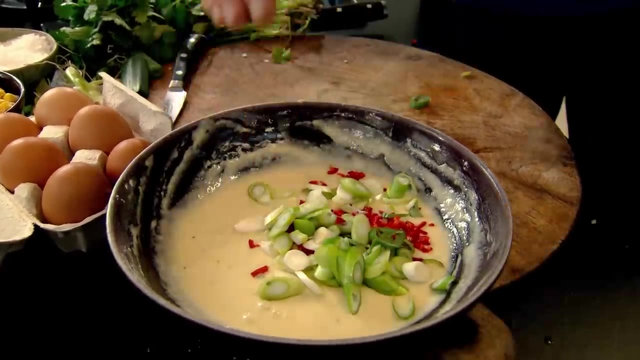 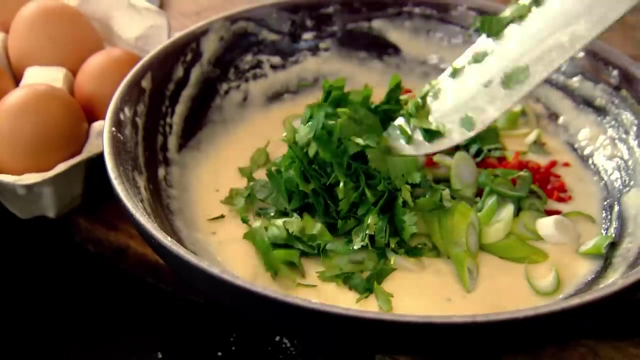 Take off that outside layer of the spring onion Top and tail, Slice at an angle So I've got a bit of texture running through the mixture. Want that nice crunch in Coriander? Just slice through Nice and gently And get that in there. 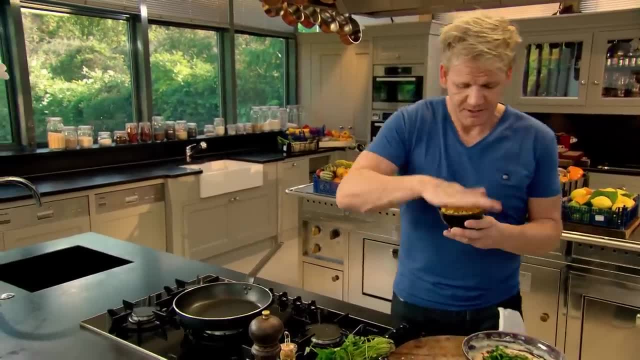 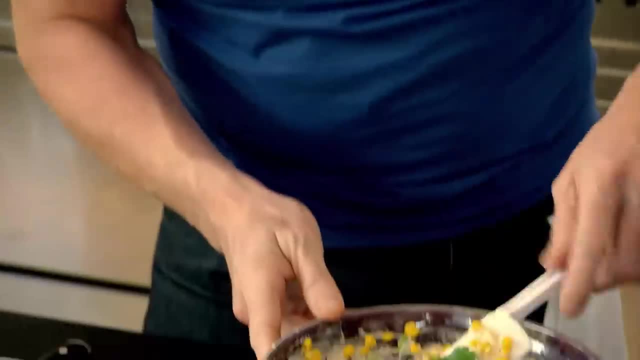 Next the sweet corn. Now drain it from the tin And just pat it dry so it doesn't make the mixture too wet. Give that a nice mix. You can see now I've got two-thirds ingredients and one-third of the mixture to bind together. 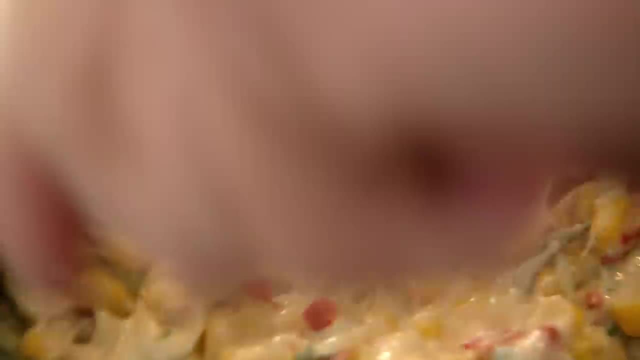 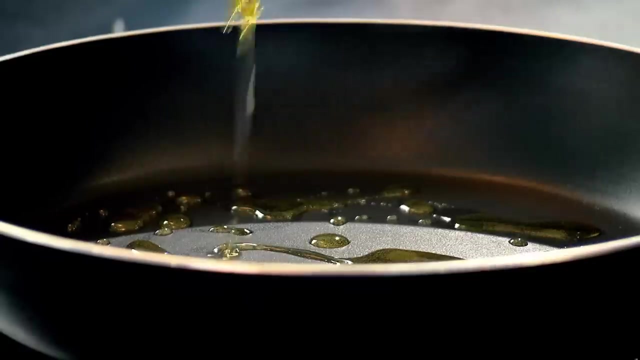 That's the secret of a good fritter. So you're biting into excitement. not sort of dough Pan on Olive oil in Nice and hot, Get a nice big dessert spoon. You know there's one nice portion. 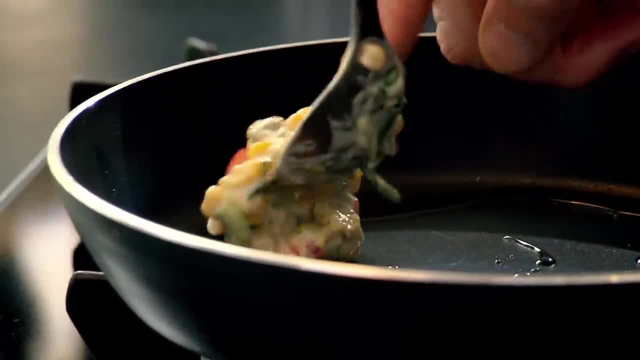 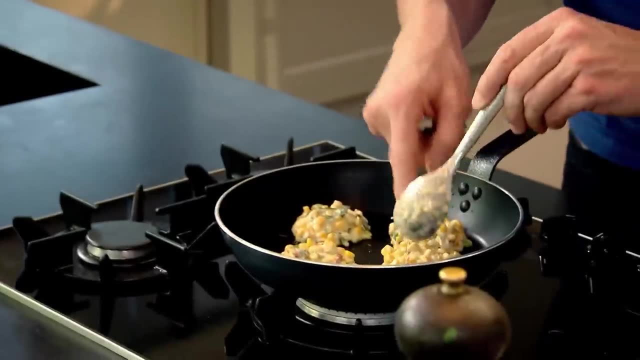 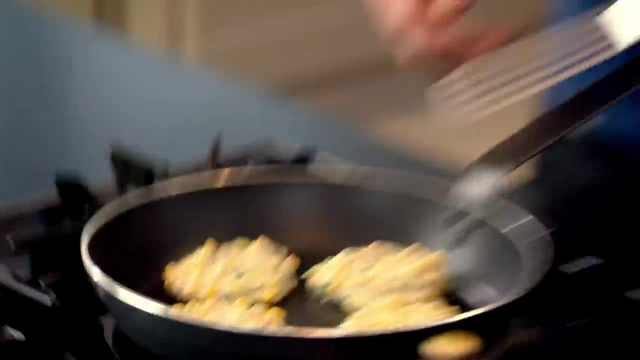 In Space the fritters evenly around the pan in a clockwise direction, so you always know which one to turn first. Just with the back of your spoon, sort of spread them out a little bit. OK, Pallet knife, Just check. 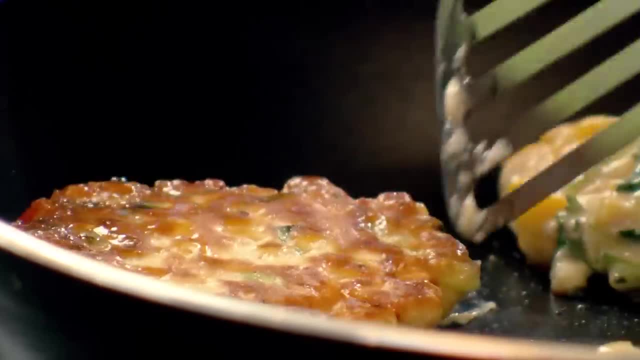 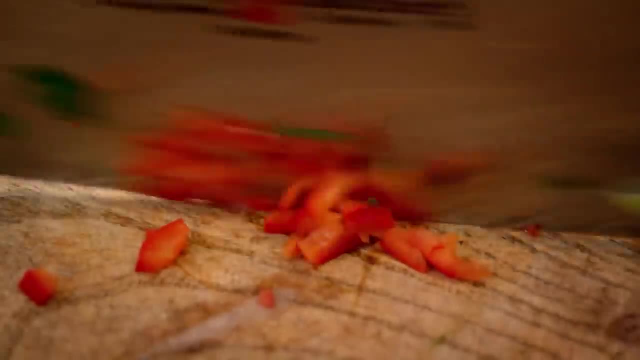 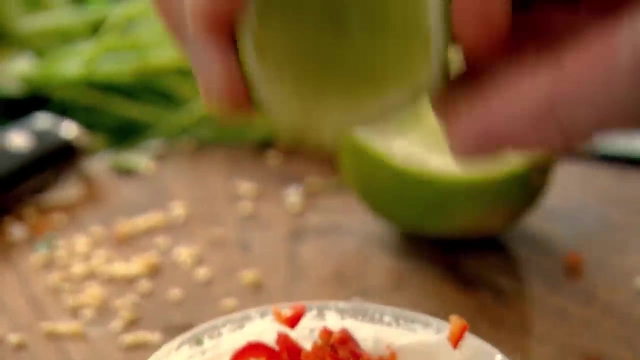 You're happy with the colour And turn over Beautiful. Now for the chilli yoghurt dressing. Deseed and finely chop a red chilli And add to a pot of natural yoghurt, And then some fresh lime.